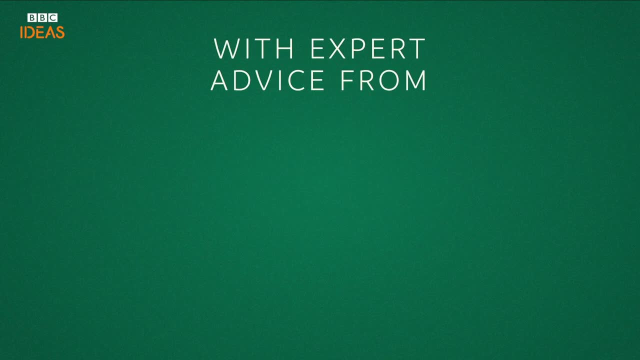 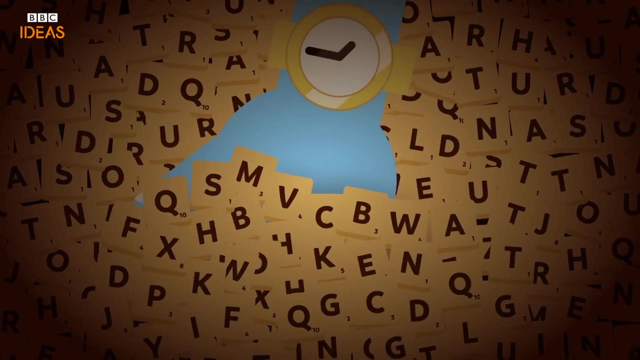 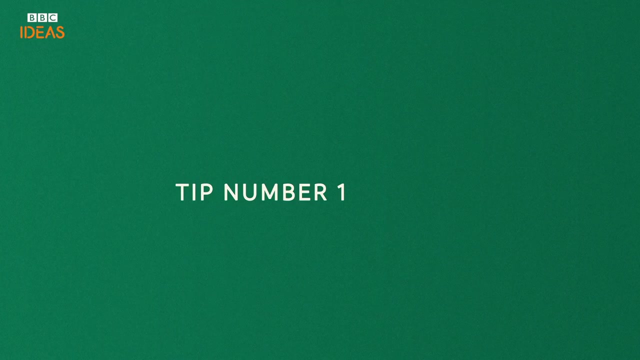 How to win at Scrabble with expert advice from Natalie Zolti. Scrabble is not just a simple word game. It requires strategy and an understanding of mathematics and probability. Here are five tips to improve your game. Tip one: learn your twos. There are 124 two-letter. 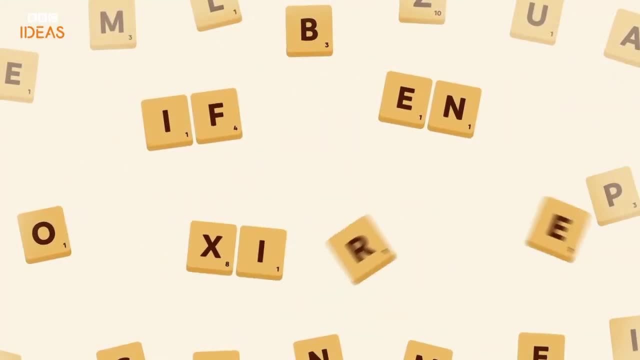 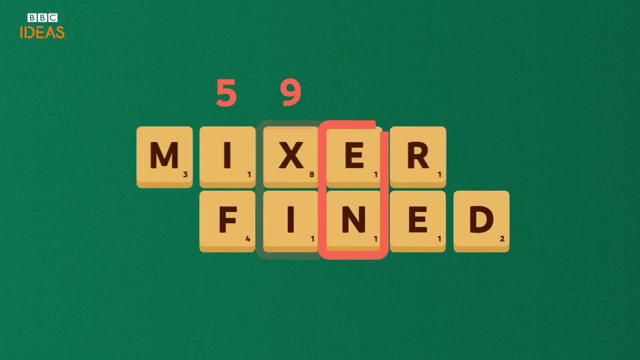 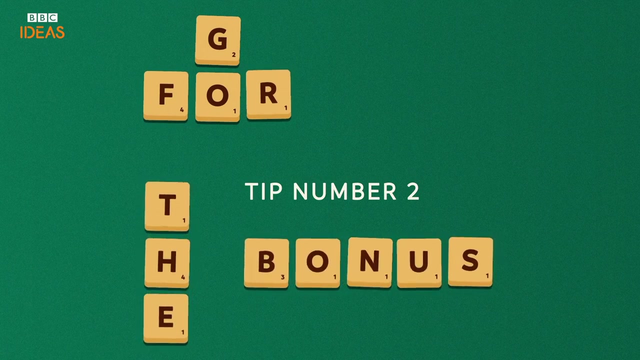 words allowed in Scrabble. Try to learn as many of them as you can, even if they look a bit weird. Then play them parallel to your opponent's word to score big points. Tip two: go for the bonus. If you play all seven letters in one turn, you get an extra 50 points. How? 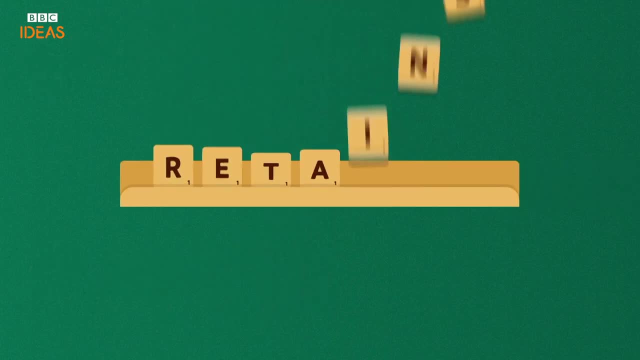 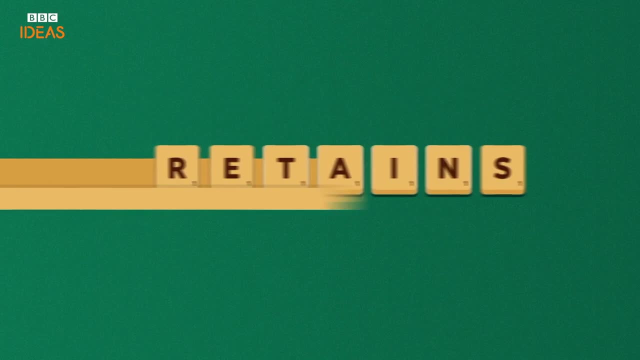 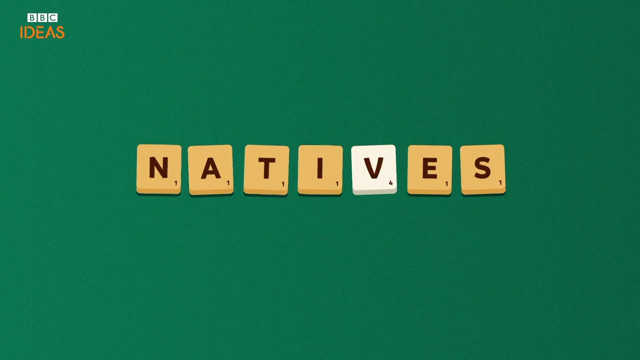 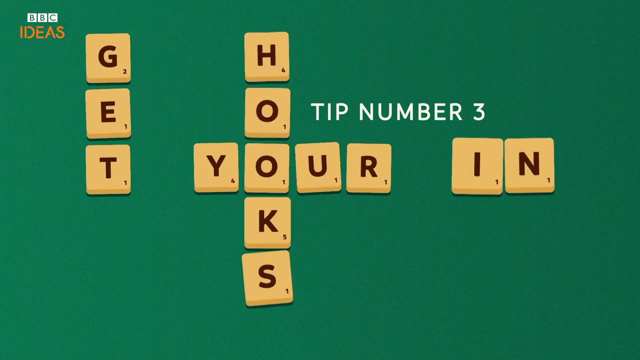 on your rack, Especially those in the word retains. These 6 letters go with every letter of the alphabet except for Q and Y to make a 7-letter word. Tip three: get your hook in. A hook is a letter that can be added to the front. 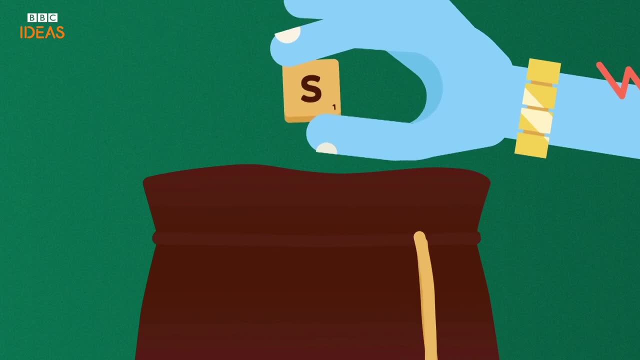 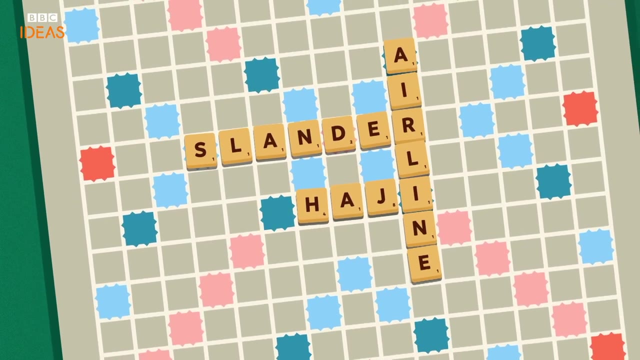 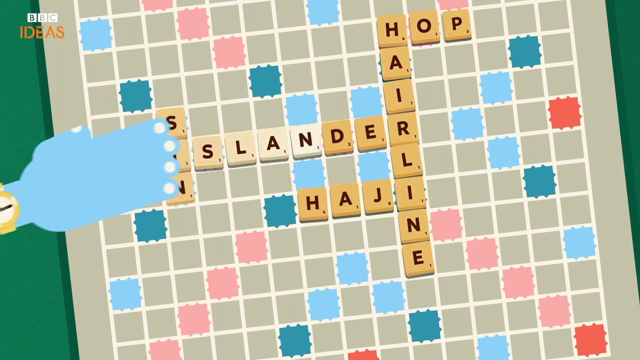 or end of the words, to make a new one. S is the most obvious, But there are many more. There are many less obvious ones you can use to surprise your opponent with a high-scoring play. Airline Hairline Slander, Islander Hodgey. 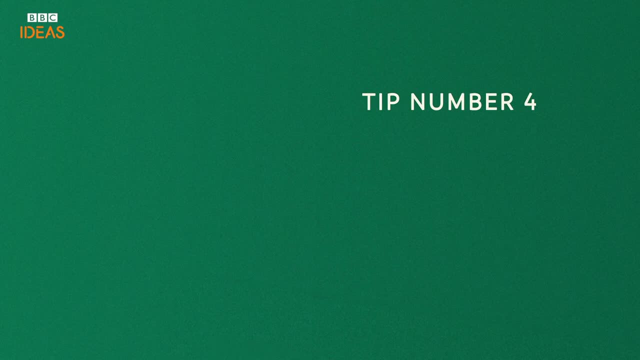 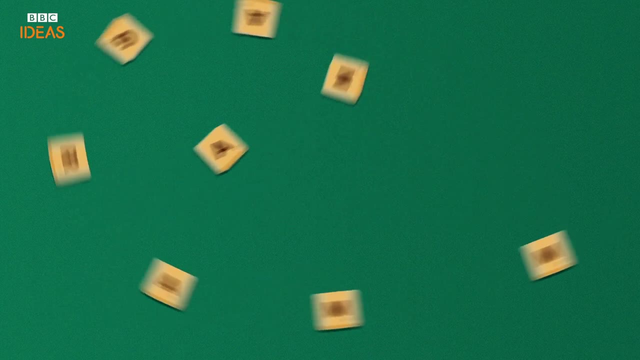 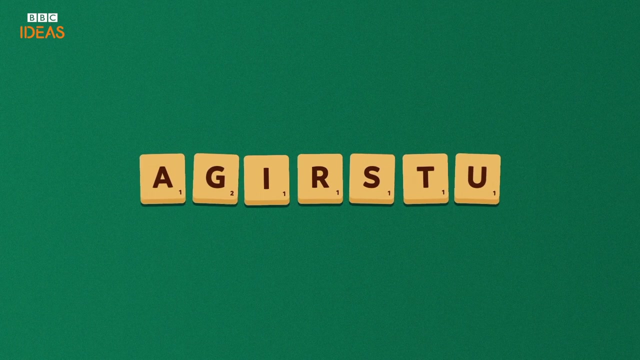 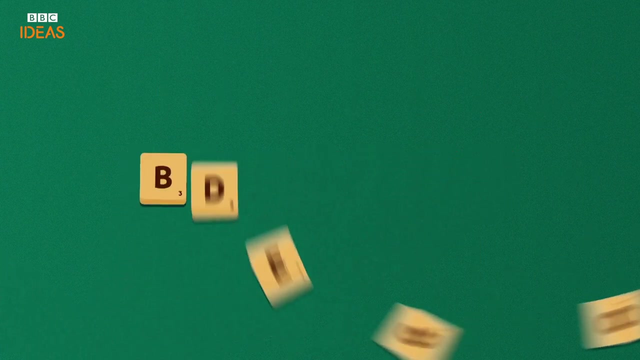 Bargy. Tip 4: Develop your anagramming muscles. Practice anagramming whenever you can. Cryptic crosswords and puzzles can help. Sometimes normal words can be surprisingly hard to spot. Egeertsu Guitars, Badegui, Goodbye. 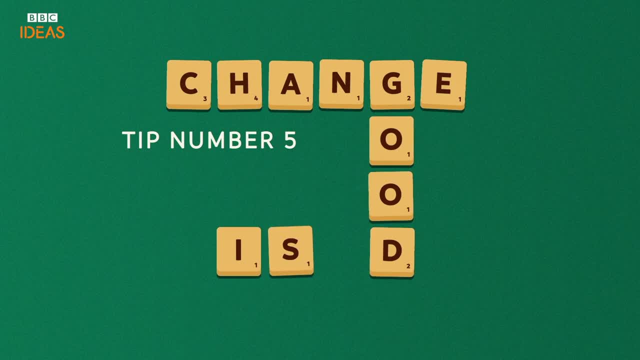 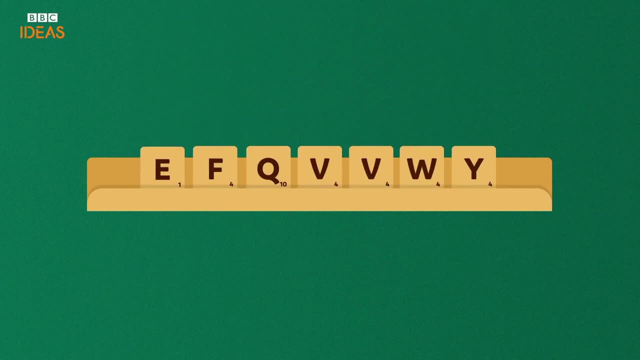 Tip 5: Change is good. Don't be frightened to exchange some or all of your tiles. rather than playing a word, It can be the best thing to do. High-scoring tips- High-scoring tiles- are not always good. From an opening rack like this, there is nothing you can usefully play.